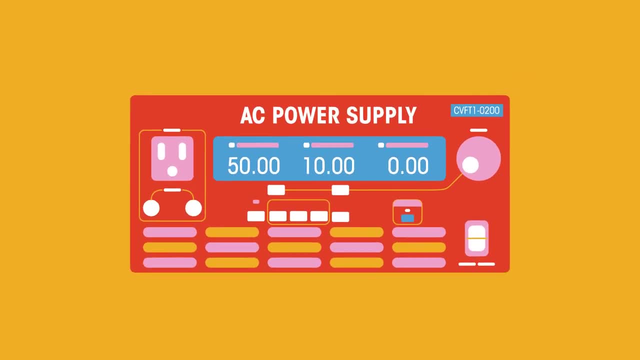 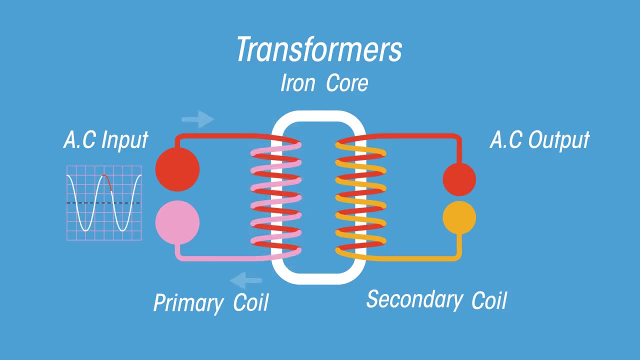 A transformer requires an alternating current or AC power supply which creates the alternating current in the first place. The alternating current passes through the primary coil wrapped around a soft iron core. This induces a changing magnetic field in the core. The changing magnetic field, like a domino effect, induces a changing magnetic current in the 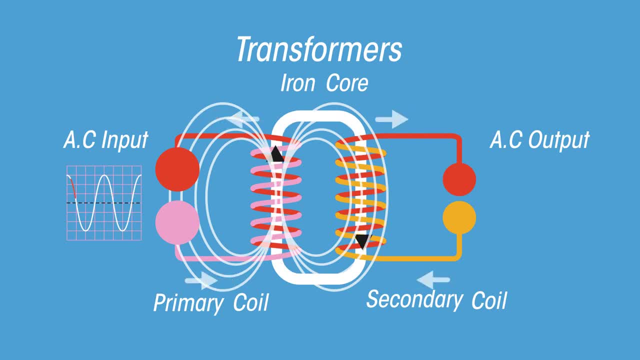 secondary coil. This alternating magnetic field in the secondary coil induces an alternating current in the circuit connected to the secondary coil. Depending on how many turns the coils on each side have, the new output will have a higher voltage than the current in the secondary coil. 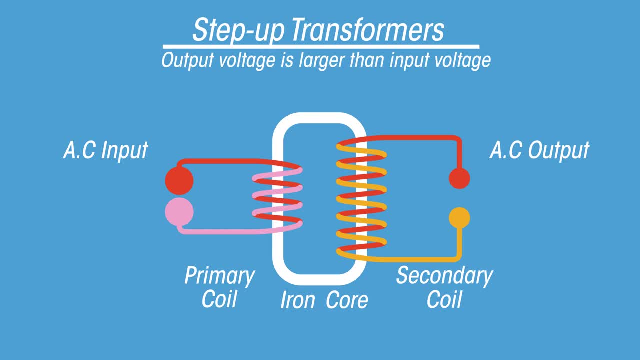 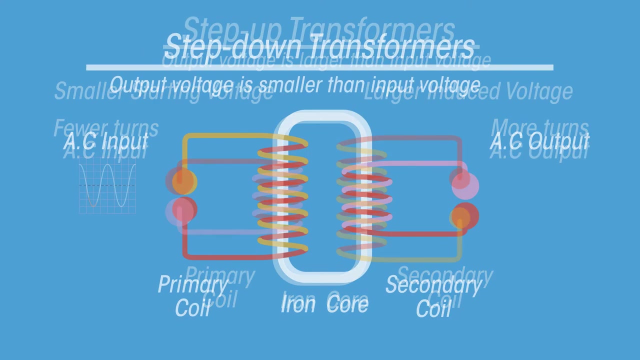 A stepped-up transformer has more turns of wire in the secondary coil than the primary coil, which in turn creates a larger induced voltage in the secondary coil. As the output voltage is larger than the input voltage, it is called a stepped-up transformer. A stepped-down transformer has more turns of wire in the primary coil. 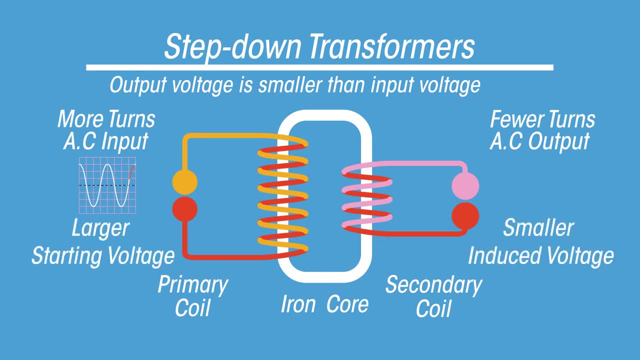 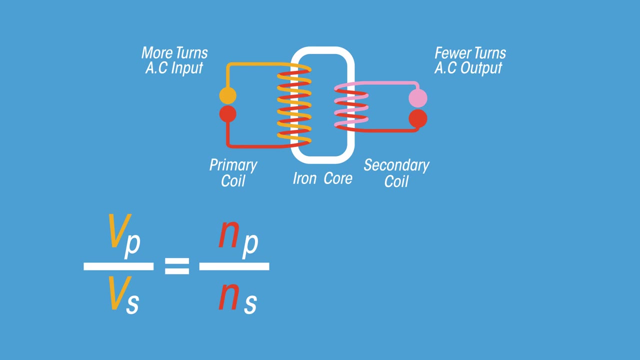 and less turns in the secondary coil. This creates a smaller induced voltage. in the secondary coil, the output voltage is smaller than the input voltage, hence it's a stepped-down transformer. We can calculate the voltage produced in the secondary coil by using this equation: the voltages in the primary and secondary coils. 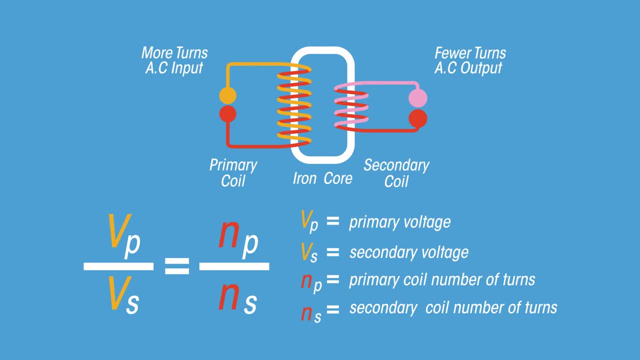 and the number of turns in each coil. So let's work out an example. Calculate the voltage in the secondary coil Using our equation. we can substitute in the values we already know. The primary voltage is thirty volts. the primary number of turns is thirty volts. the primary voltage is thirty volts. 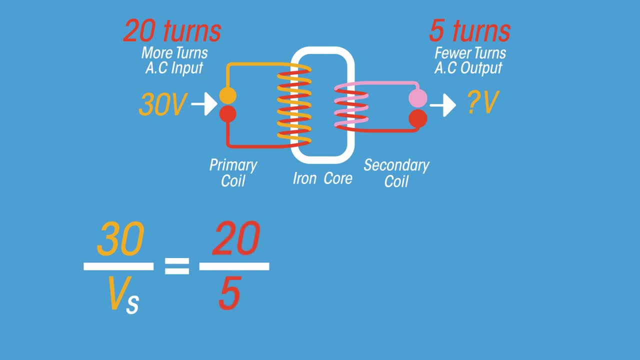 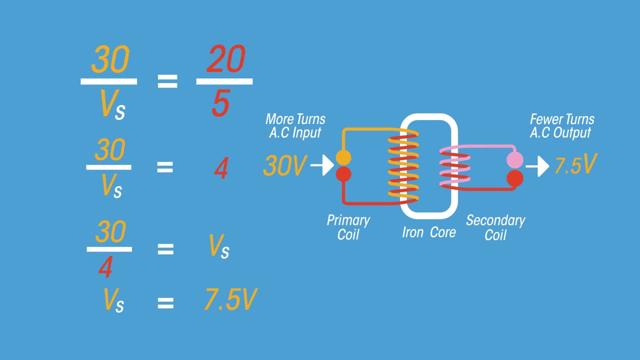 turns is 20 and the secondary turns is 5.. A simple bit of rearranging. and the secondary voltage is 7.5 volts. So the output voltage of 7.5 is less than the original supply of 30 volts. Is this a step up or a step down? transformer A. 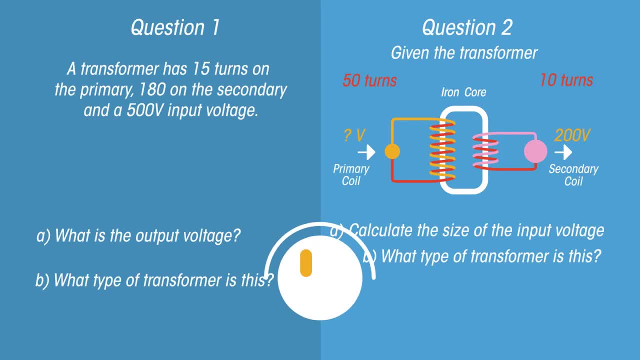 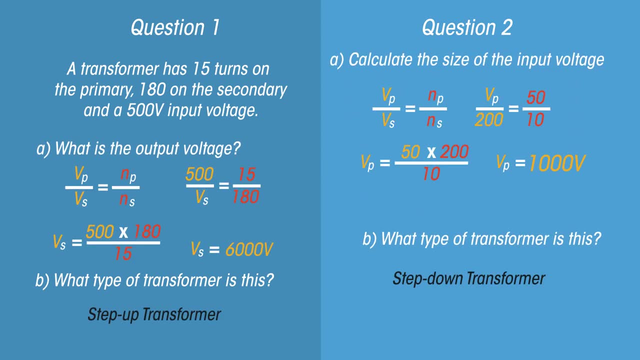 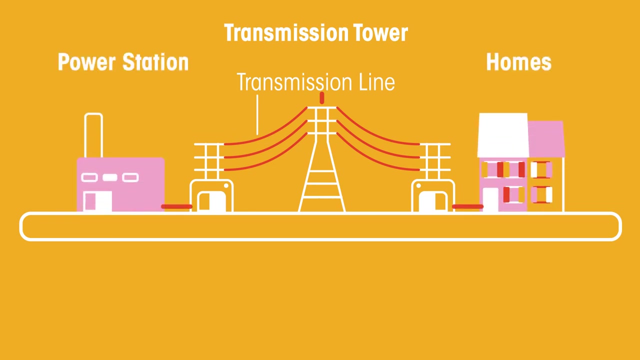 step down, of course. Pause the video and give these questions a go. Did you get them right? A 6,000 volt step up transformer and the step down transformers start with a thousand volts. Transformers are used in the real world in the transfer of electricity from power stations to our homes. When a